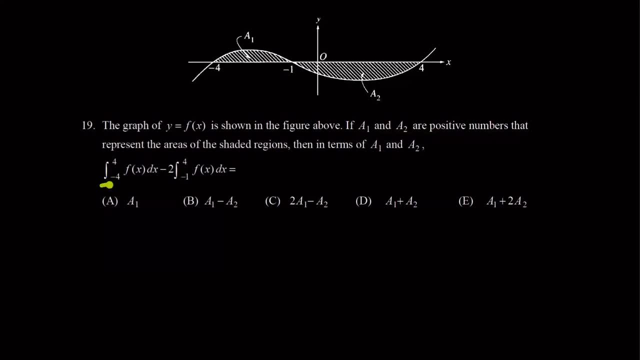 And so we are being asked to evaluate the difference of these two integrals terms of the areas a1 and a2.. And let's start with the first integral. The first integral is integral from negative 4 to 4, f of x, dx, And we can break it into two integrals from negative 4. 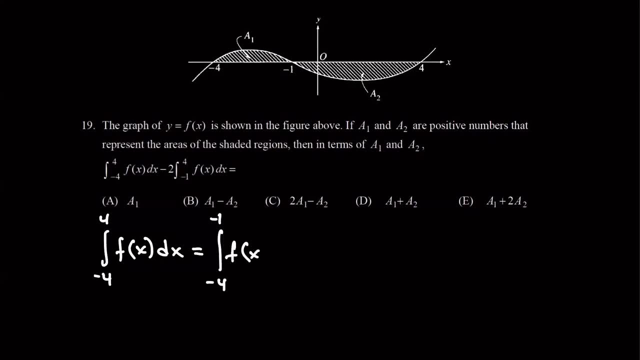 to negative 1, f of x dx, plus an integral from negative 1 to 4, f of x dx, And recall that the integral is actually the area under the curve. So, for example, for the first integral the area is equal to a1 and it is positive, So the first integral is equal to a1.. 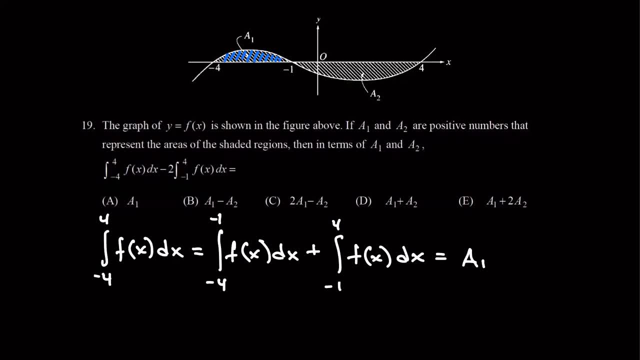 The second integral is equal to the area under the curve, but it is in this case negative because the curve lies under the x-axis. So this is equal to in terms of the area, this is equal to negative a2.. So let's now look at the second integral. It's an integral from negative 1 to 4, f of x, dx. 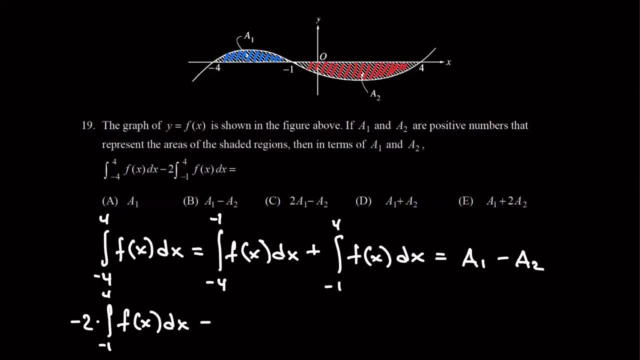 And we have to multiply by negative two. up front, This is equal to negative two and that, as we just said, it's negative a2, the second area. So multiplying gives us two a2.. So overall, getting back here, we can plug in now the expressions a1 minus, a2 for the first integral plus. 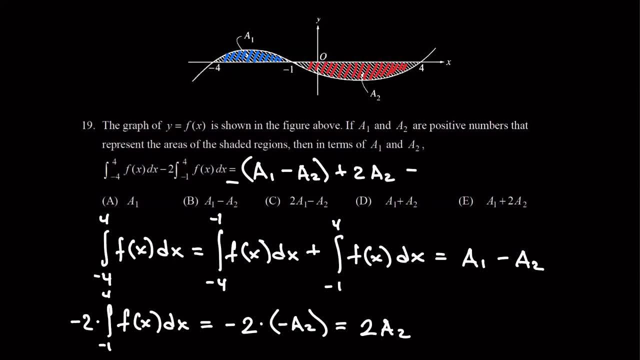 two a2 for the second integral, This is equal to a1 plus a2.. Looking at the possible answers, we see that the answer is d, a1 plus a2.. So what did we learn here is that the area under the curve for the integral is equal to the area. 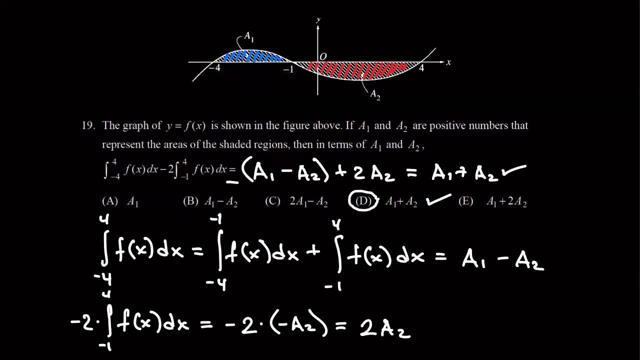 under the curve and so it's positive when the curve is above x-axis and it's negative when the curve is below x-axis. And the rest is also remembering that the integral itself is an area under the curve. So this integral here is an area under the curve and this integral here